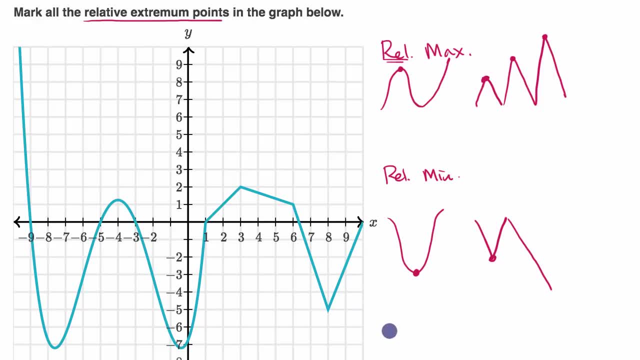 and relative minima, and that's where the graph is flat. So if you have parts of your function where it's just constant, these points would actually be both. For example, if this is our x-axis, right over here, that's our x-axis. 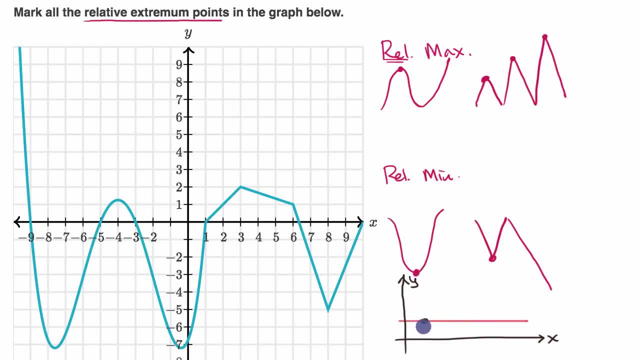 If this is our y-axis right over there, and if this is x equals c. if you construct an open interval around c, you notice that the value of our function at c, f of c, is at least as large as the values of the function around it. 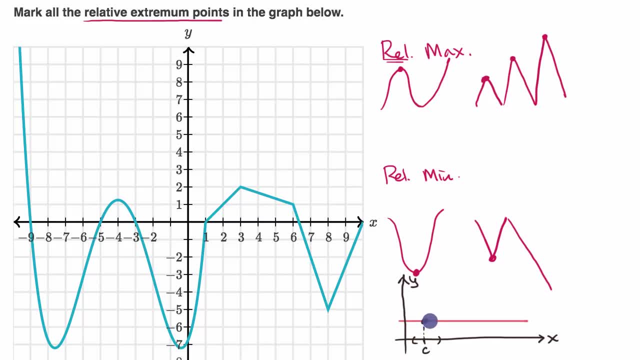 And it is also at least as small as the values of the function around it. So this point would also be considered a relative minimum point. But that's an edge case that you won't encounter as often. So with that primer out of the way, 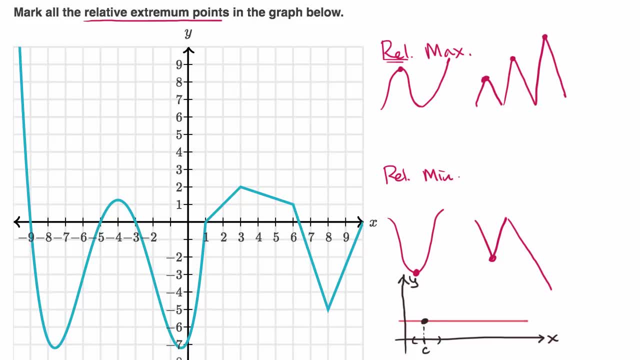 let's identify the relative extrema. So first the relative maximum points. Well, that's the top of a hill right over there. This is the top of a hill. You might be tempted to look at that point and that point. but notice, at this point right over here. 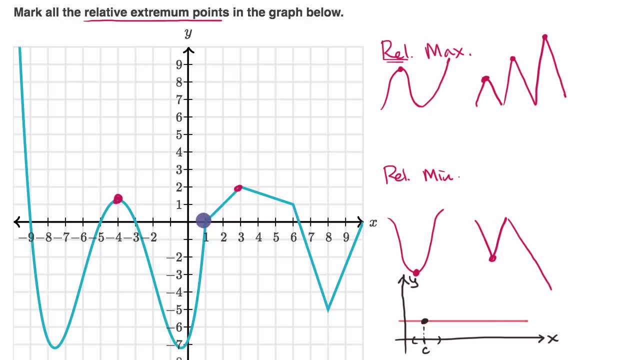 if you go to the right, you have values that are higher than it, So it's really not at the top of a hill. And right over here, if you go to the left, you have values that are higher than it, So it's also not the top of a hill. 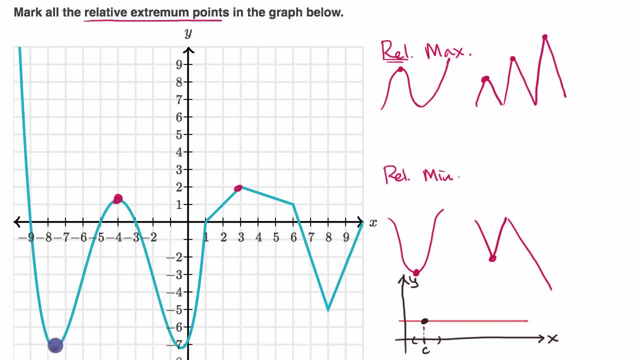 And what about the relative minimum points? Well, this one right over here is a relative minimum point, This one right over here is a relative minimum point And this one over here is a relative minimum point. Now let's do an example dealing with absolute extrema. 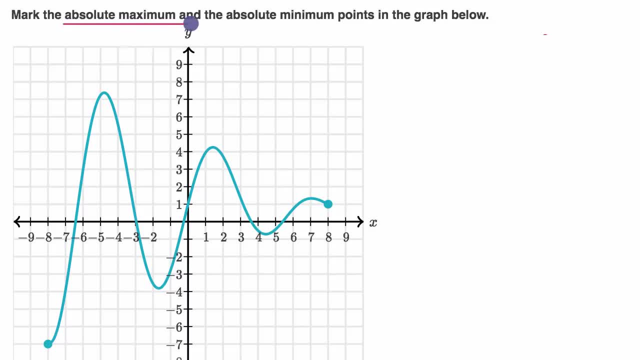 So here we're told to mark the absolute maximum and the absolute minimum points in the graph below. So once again, pause this video and see if you can have a go at this. So you have an absolute maximum point at, let's say, x equals c, if, and only if, 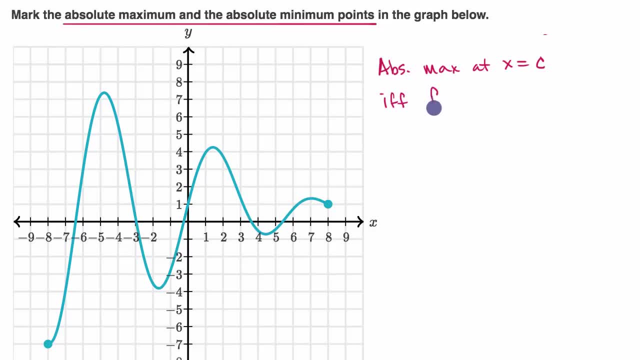 so I'll write if, for if, and only if, f of c is greater than or equal to f of x for all the x's in the domain and you have an absolute minimum at x equals c, if, and only if if, f of c is less than or equal to f of x.